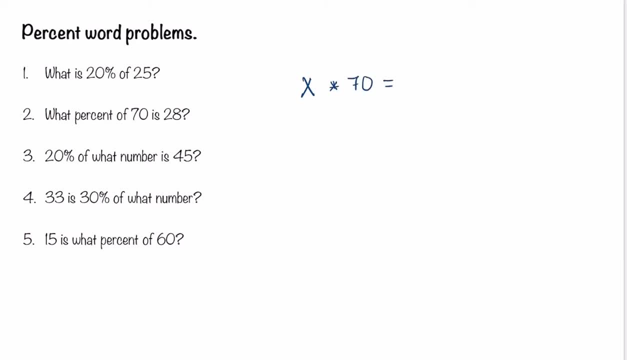 70 is is equal to 28.. Now here we need to divide by 70 on both sides to get x. x is going to equal to. We're going to divide the top by 7.. That gives us 4, 10.. 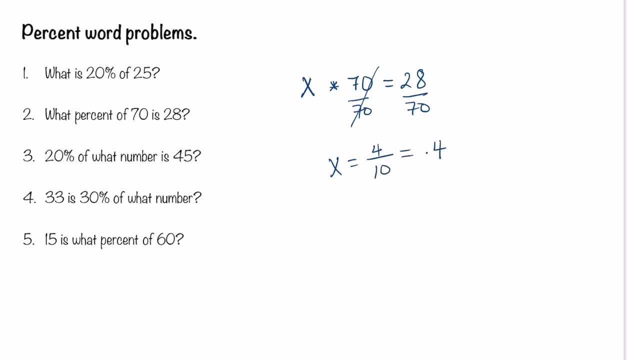 4 divided by 10 is 0.4.. 0.4 is equal to 40%, And so here's our answer on this one, which is 40%, And I need to write the answer for the last one, which is 5.. 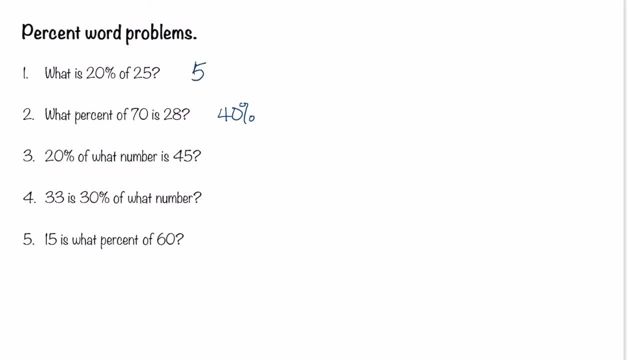 Number three: 20% of what number is 45?? By now you should know that when you have the word of, that means multiply. What number is an unknown We're going to use x? Is is equal to, So let's write this: 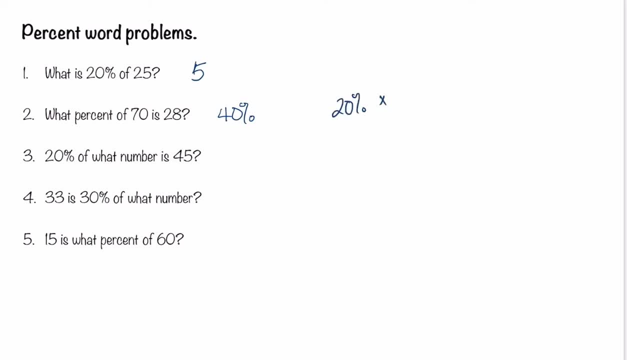 20% of times what number x is, 45. Is is equal to, and 45. Now we're going to divide both sides by 20% And here we have: x is equal to 45 divided by 20%. This can be confusing. 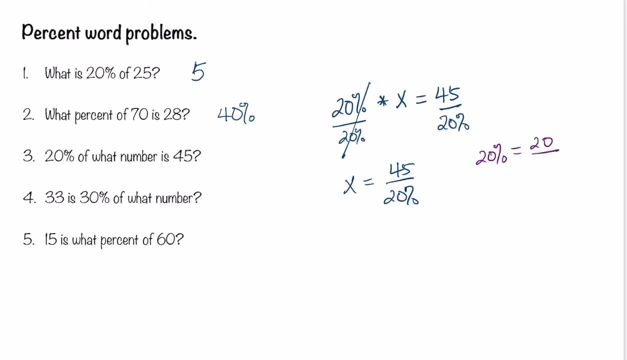 20% is the same as 20 divided by 100. Now we're going to substitute that into this equation. 20% becomes 20 divided by 100. The same as 45 times the reciprocal of the denominator, And that is 100 divided by 20.. 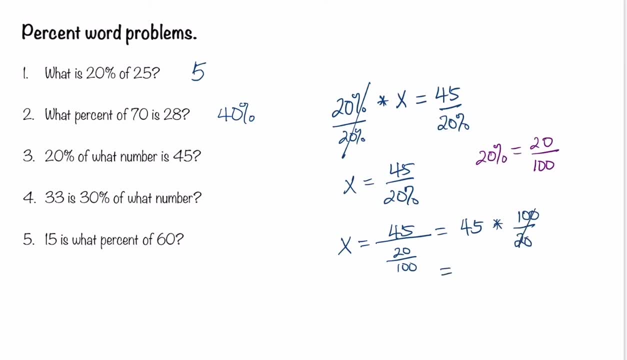 And here we get: 5 times 45 is equal to 225.. So we have: x is equal to 225.. Number four, 33 is 30% of. what number? We're going to write this into an equation? 33 is is equal to 30% of is multiply what number x. 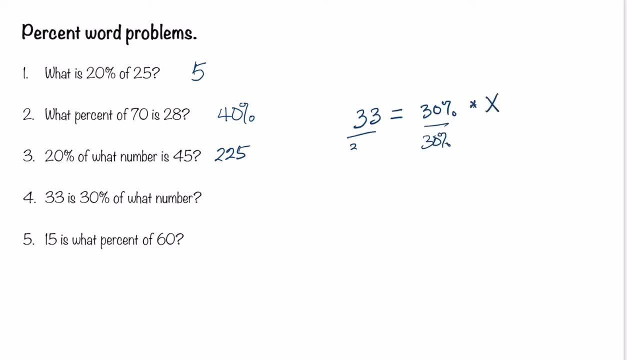 To solve for x. we're going to divide by 30%. This will cancel, And the 30% We're going to change that into a fraction. 30% is equal to 30 over 100.. We're going to use that substitution. 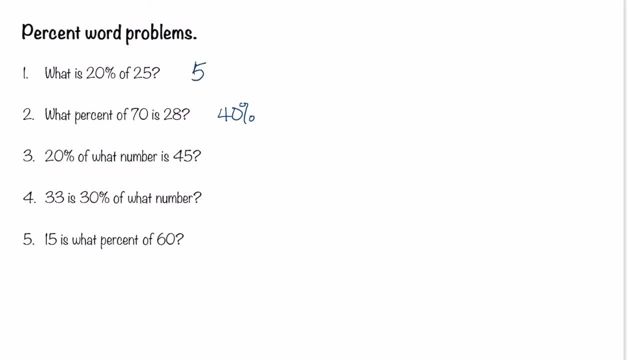 Number three: 20% of what number is 45?? By now you should know that when you have the word of, that means multiply. What number is an unknown We're going to use x? Is is equal to, So let's write this: 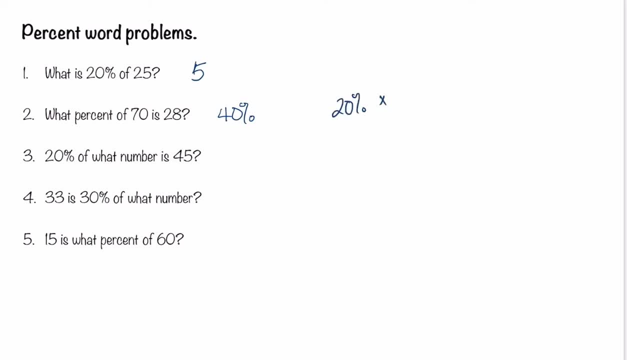 20% of times what number x is, 45. Is is equal to, and 45. Now we're going to divide both sides by 20% And here we have: x is equal to 45 divided by 20%. This can be confusing. 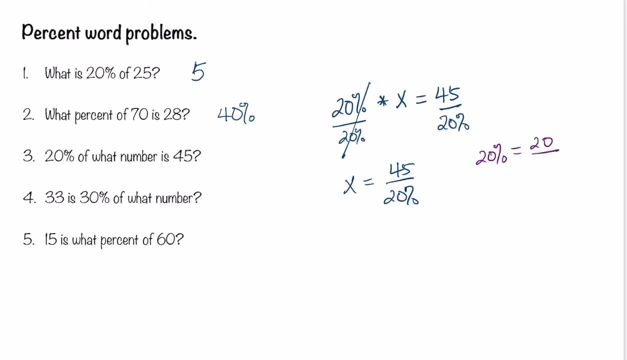 20% is the same as 20 divided by 100. Now we're going to substitute that into this equation. 20% becomes 20 divided by 100. The same as 45 times the reciprocal of the denominator, And that is 100 divided by 20.. 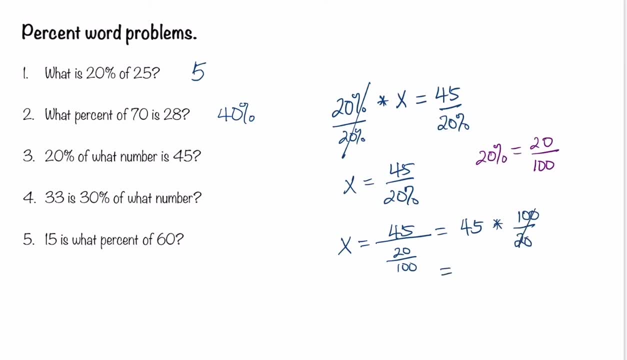 And here we get: 5 times 45 is equal to 225.. So we have: x is equal to 225.. Number four, 33 is 30% of. what number? We're going to write this into an equation? 33 is is equal to 30% of is multiply what number x. 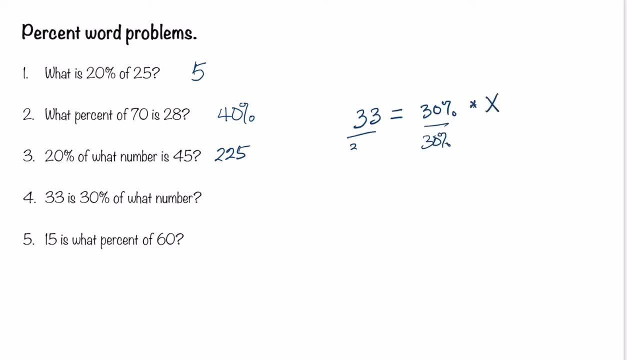 To solve for x. we're going to divide by 30%. This will cancel, And the 30% We're going to change that into a fraction. 30% is equal to 30 over 100.. We're going to use that substitution. 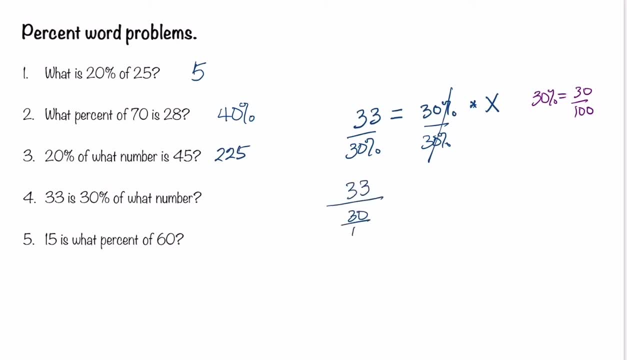 It becomes 33 divided by 30 over 100. Which is equal to 33.. Times the reciprocal of the denominator, It becomes 100 divided by 30.. We're going to cancel the 0 out And then we're going to divide the numerator. 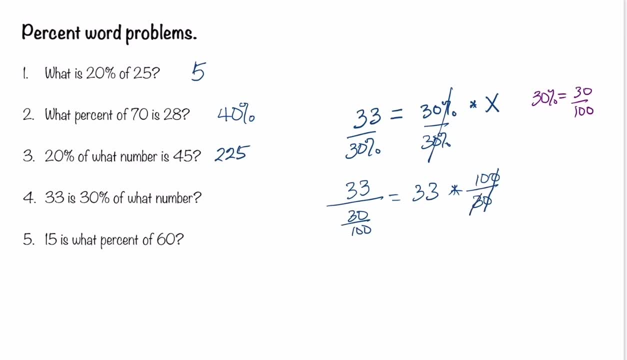 And the denominator by 3. This becomes 1., This becomes 11.. So 11 times 10. Is 110.. And that's our answer right here: 110.. Now let's do our final problem: 15 is what percent of 60..